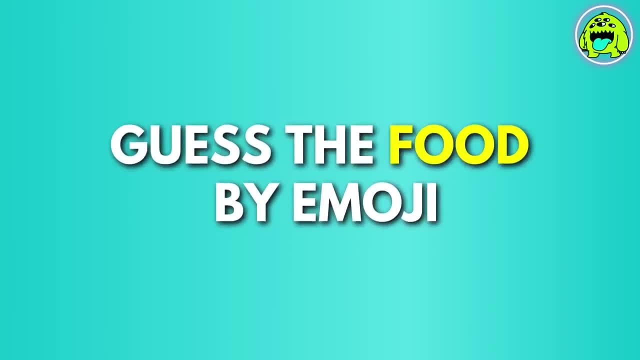 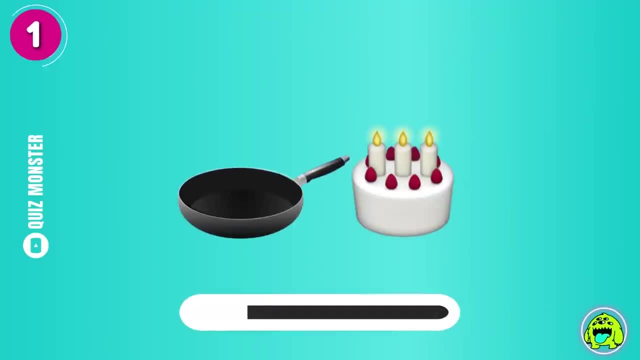 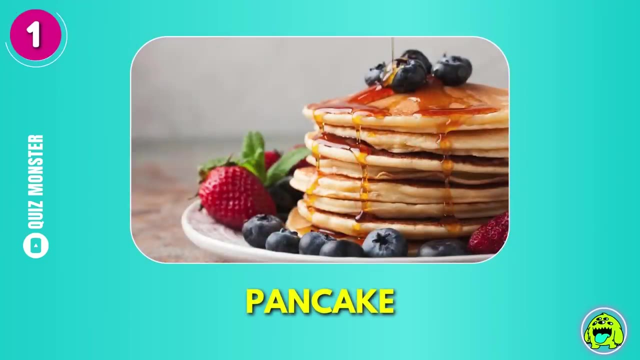 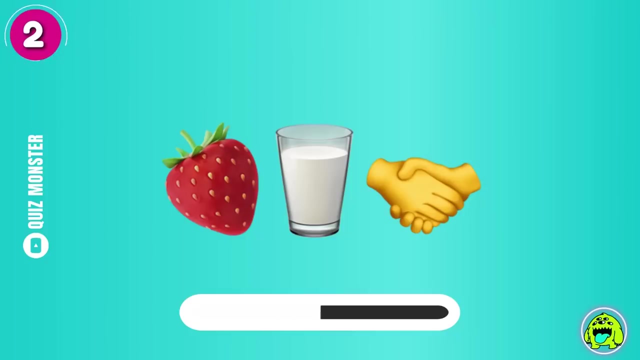 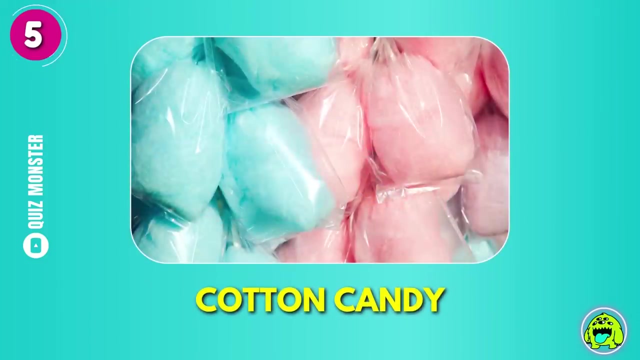 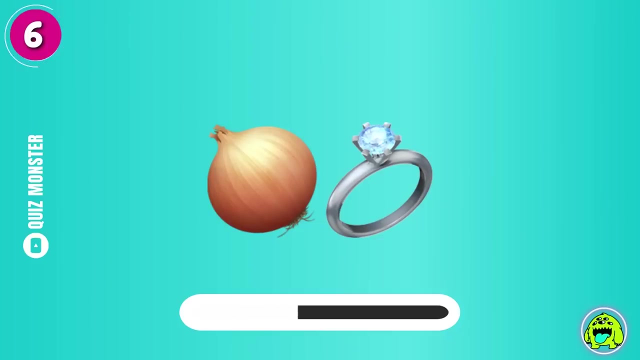 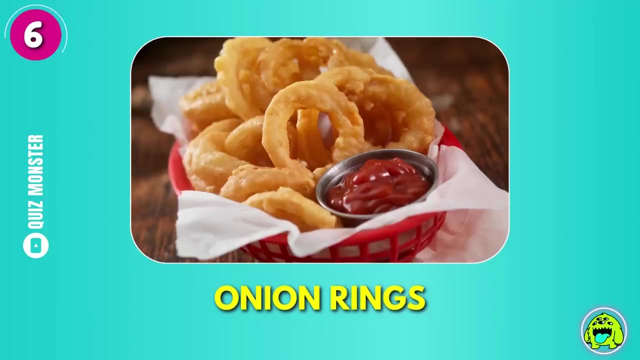 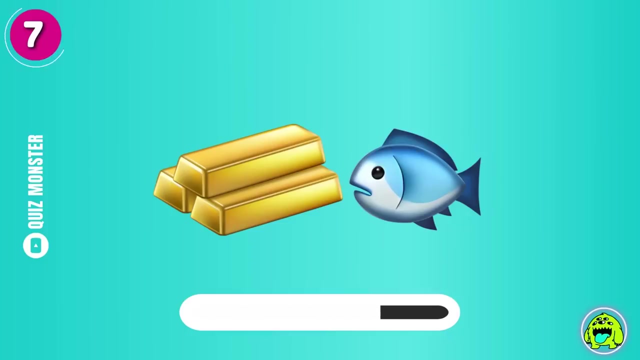 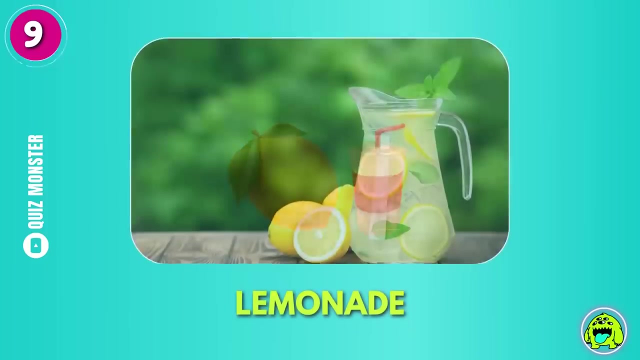 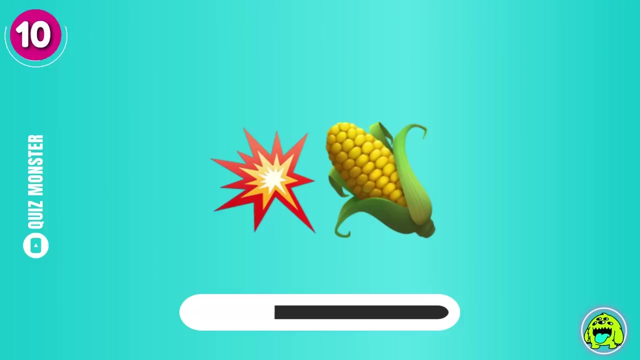 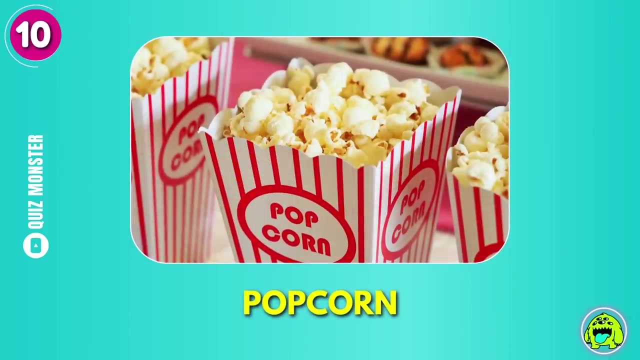 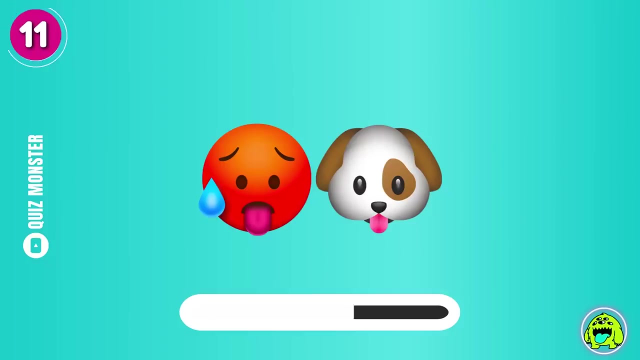 Hey Monsters. Let's guess the food by emoji. Let's go: Pancake, Strawberry, Milkshake, Gummy Bears, French Fries, Cotton Candy, Onion Rings, Goldfish, Moon Pie, Lemonade, Popcorn, Hot Dog. 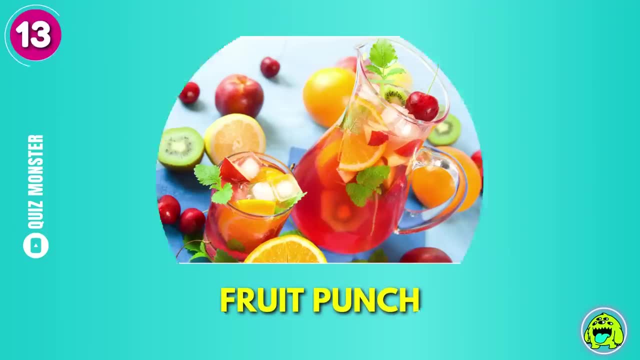 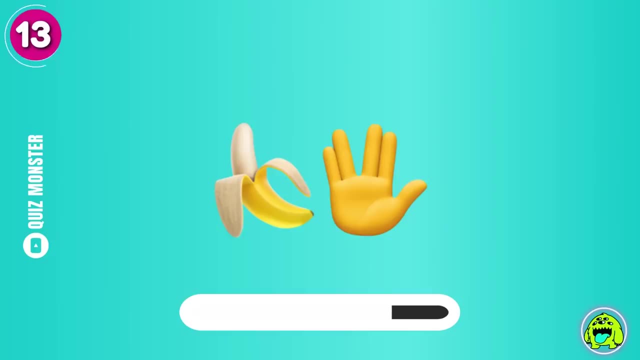 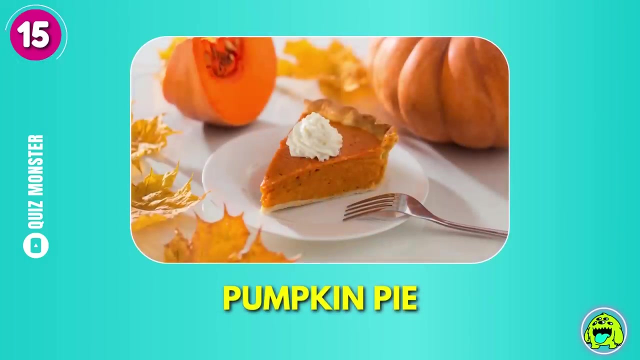 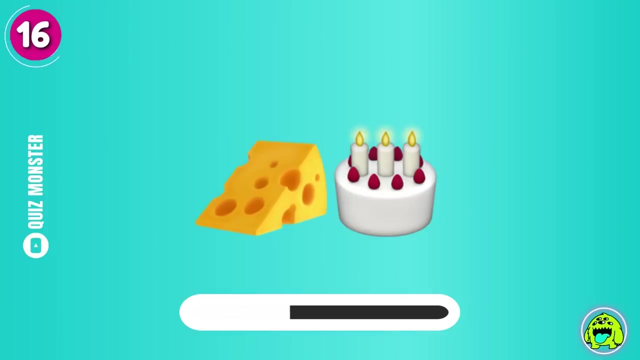 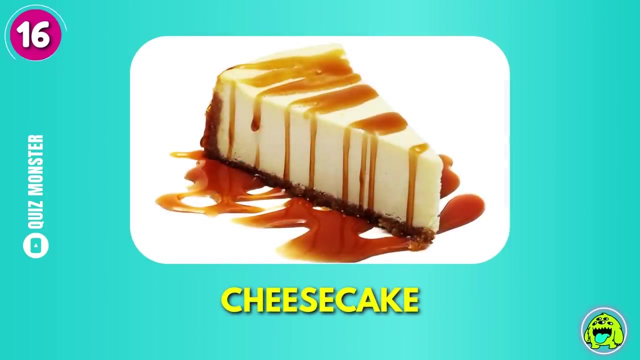 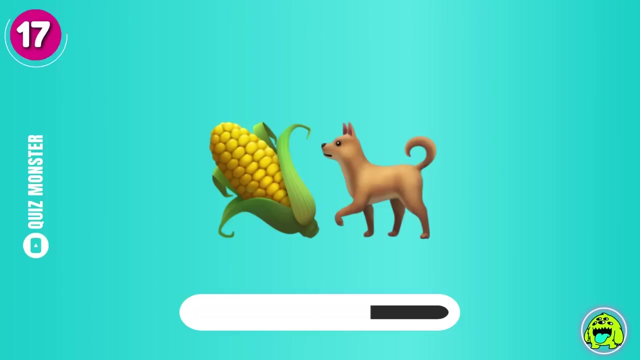 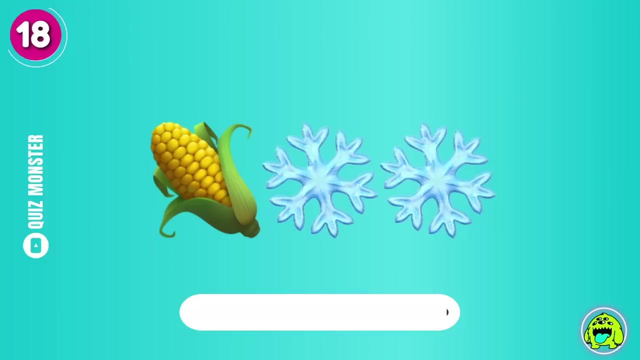 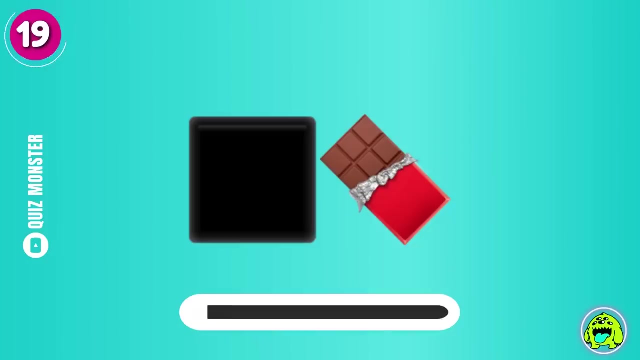 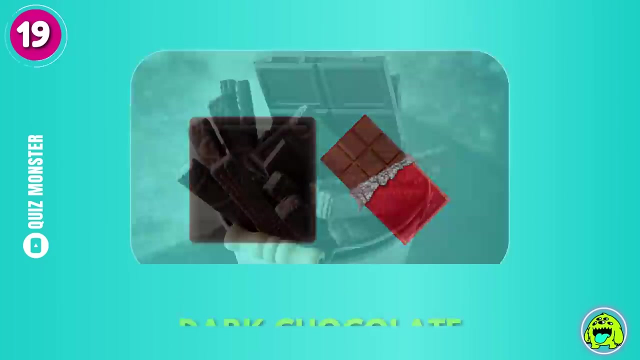 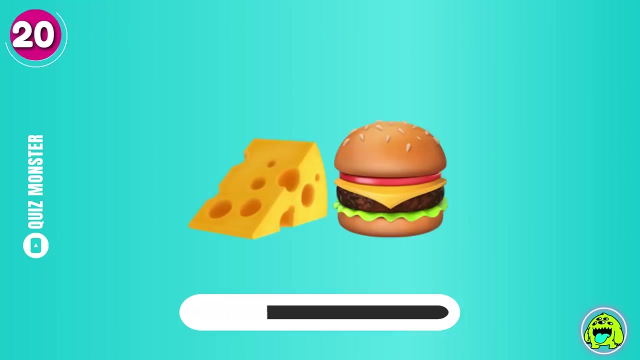 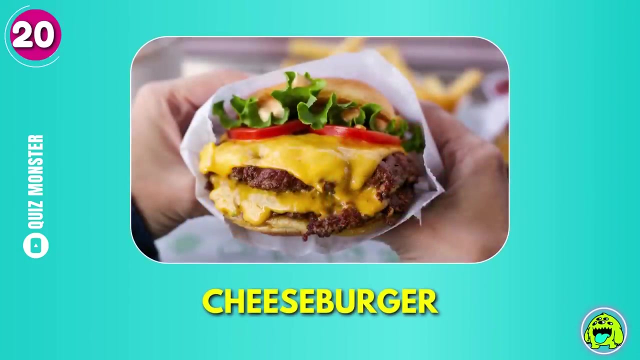 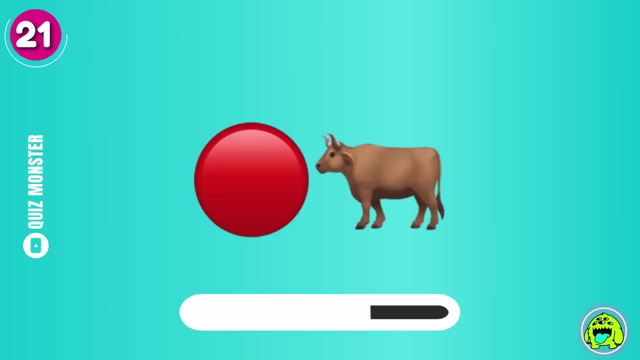 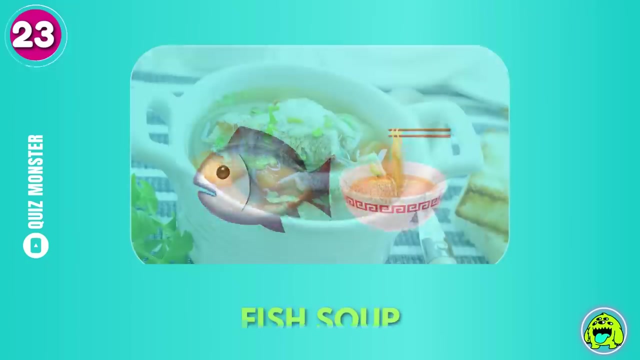 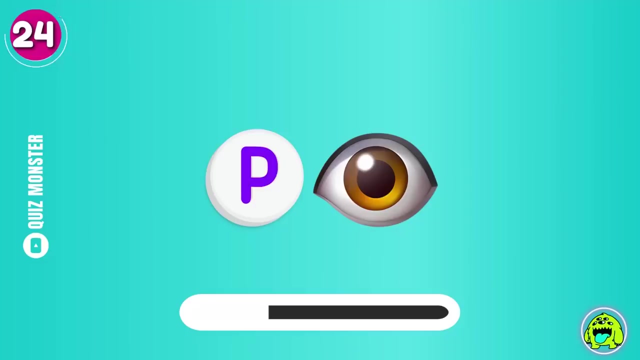 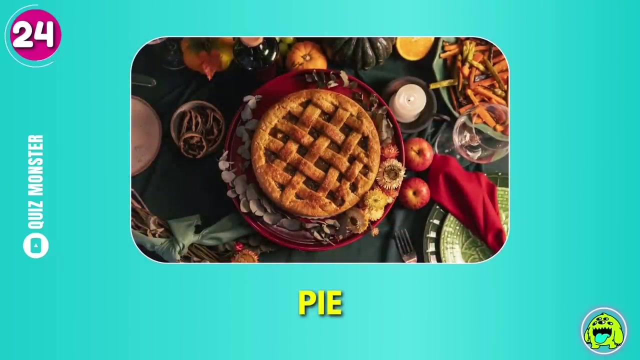 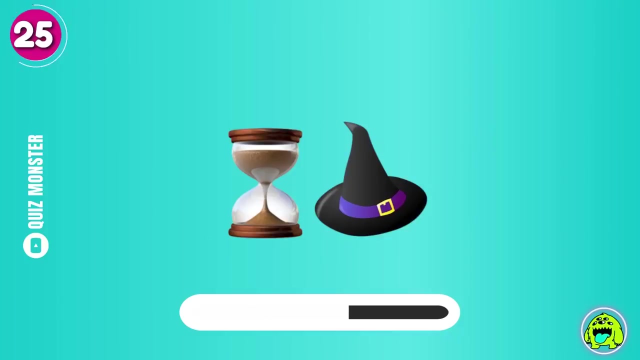 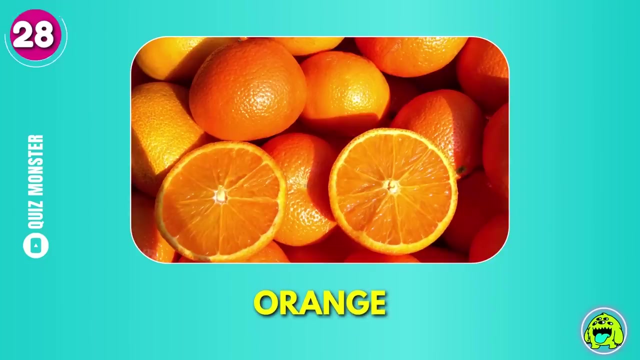 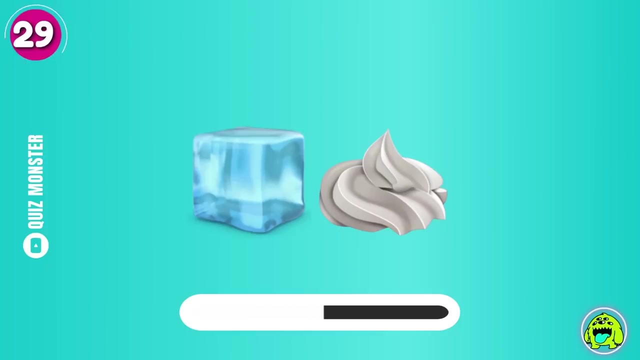 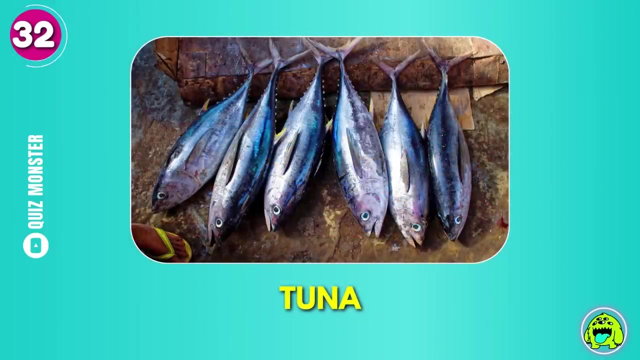 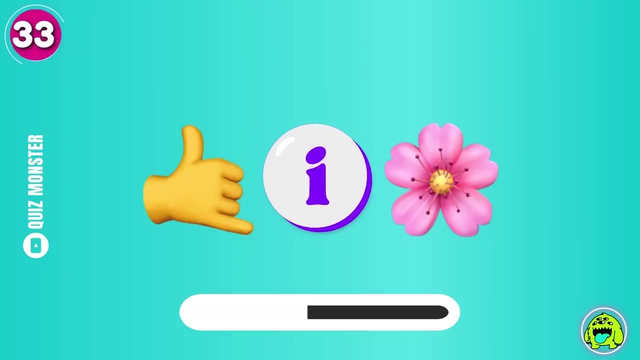 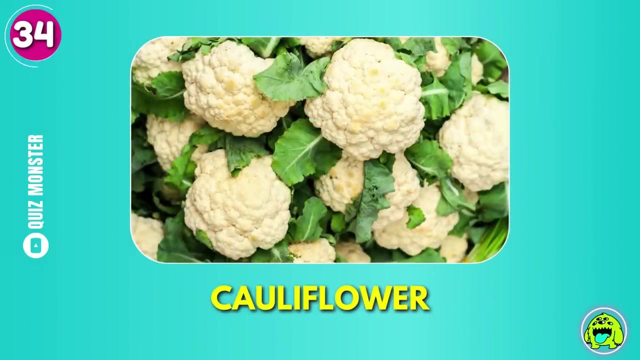 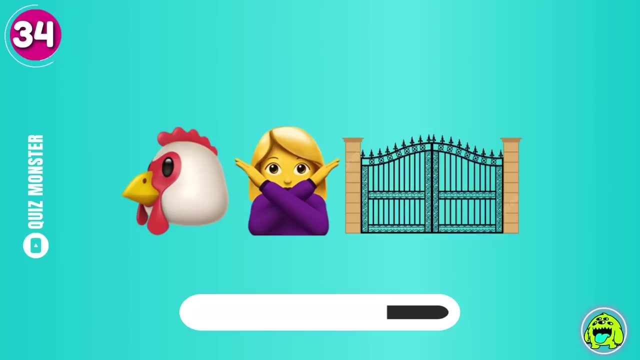 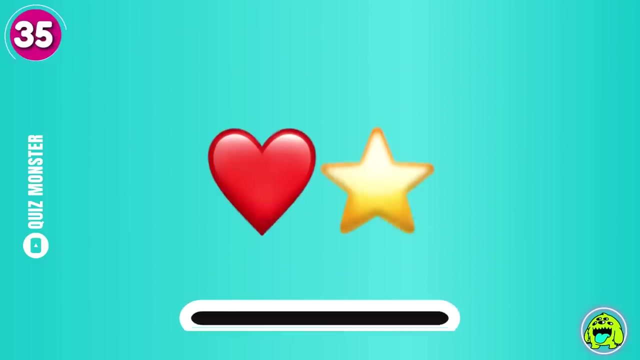 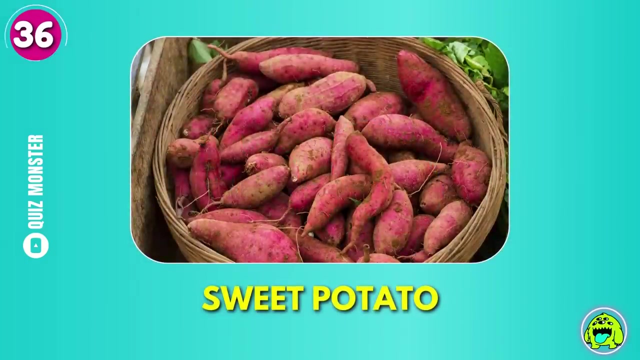 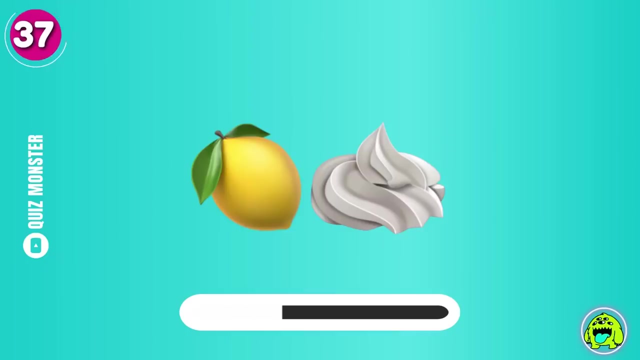 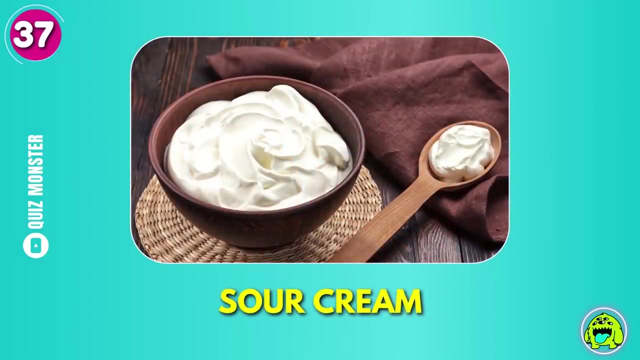 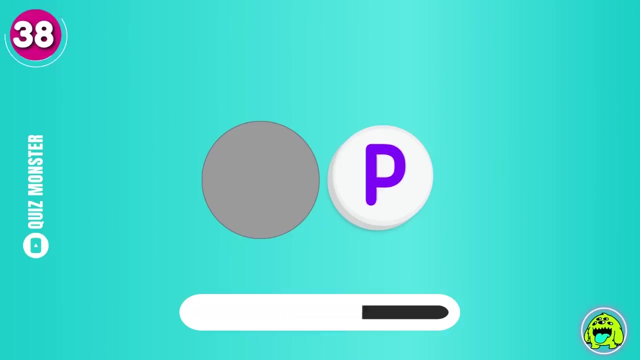 Red Bull Sushi, Sushi fish soup pie, sandwich, tomato, olive oil, orange, ice cream, bread, butter, butter, tuna, tuna, butter, maize, flour, flour, flour, flour, flour, bitc, big Lobster, Sweet potato, Sour cream, Grape, Grapes, Meatball, Carrot.